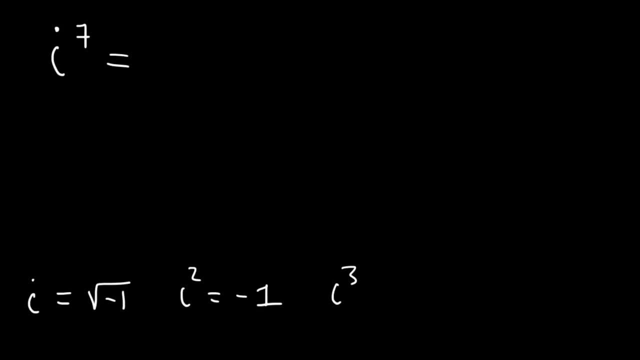 i squared is negative 1.. i to the 3rd i cubed is basically: i squared times i And i squared is negative 1, so negative 1 times i is simply negative i. So that's i cubed. i to the 4th. i to the 4th is basically: i squared times i squared. 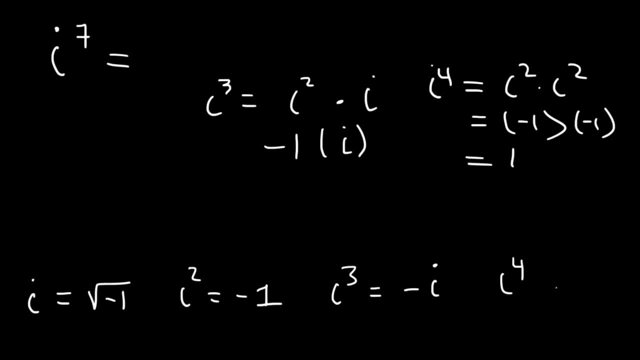 And i squared is negative 1.. Negative 1 times negative 1 is 1.. So i to the 4th is 1.. Make sure you know these four values. The ones that you're going to be using are i squared, i cubed and i to the 4th. 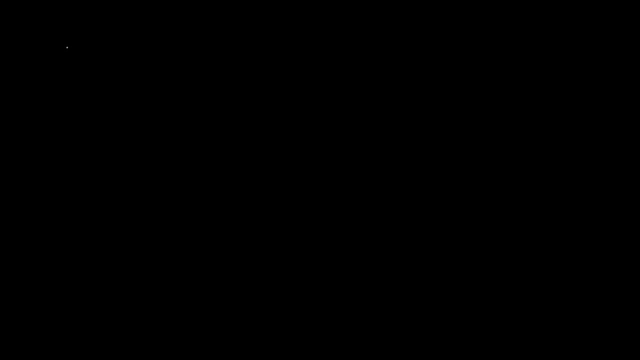 So now let's simplify: i to the 7th power, i to the 7th is i to the 4th times i to the 3rd, Because 4 plus 3 adds up to 7.. Now we know that i to the 4th is 1.. 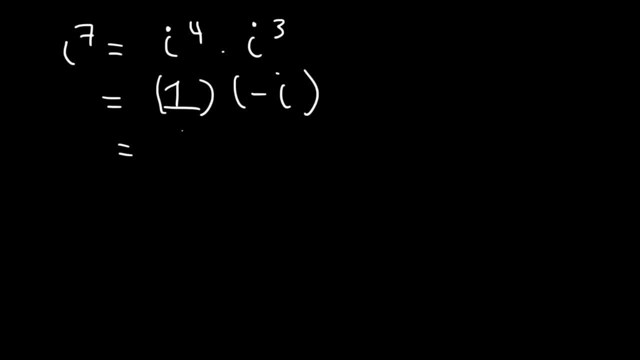 And i to the 3rd is negative. i Therefore i to the 7 simplifies to negative. i Try this one Simplify. i to the 21st power. Feel free to pause the video and work on this example. So this is i to the 20th times. i to the 1st power. 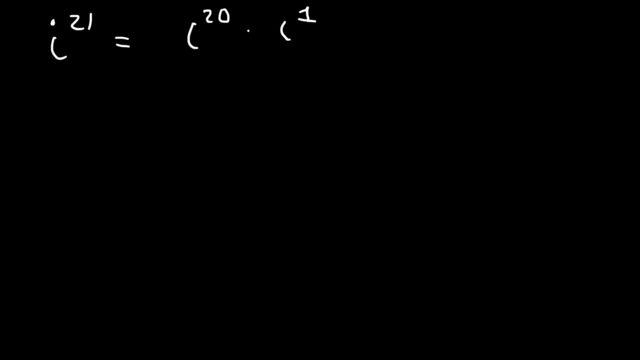 Now, the reason why I chose to separate into 20 and 1 is because 20 is a multiple of 4.. In fact, it's the highest multiple of 4, just under 21.. This one, one of them. you want it to be anywhere between 1 and 3.. 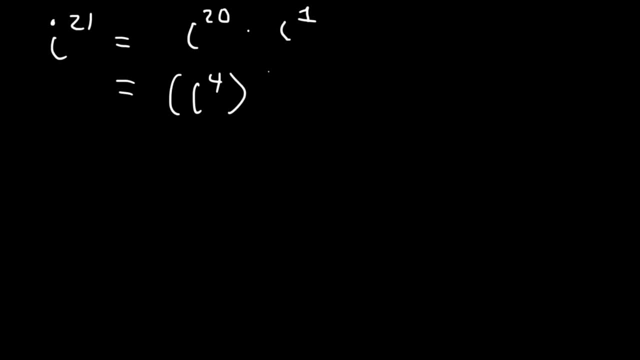 Now i to the 20th is basically i to the 4th. So i to the 4th raised to the 5th power, Because 4 times 5 is 20.. And i to the 4th, we know it's 1.. 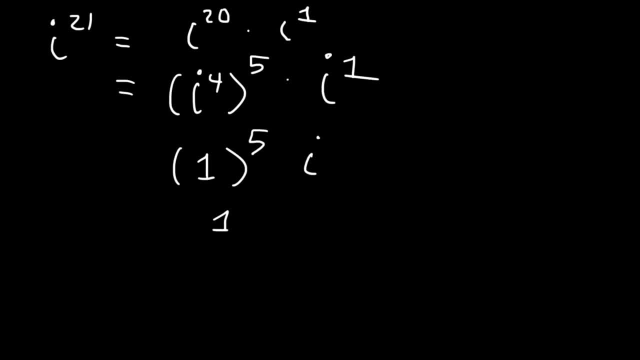 And 1 to the 5th power is simply 1.. So the answer is 1 times i, which is equal to i, And so that's the answer. Here's another one that you could try. Try i raised to the 42nd power. 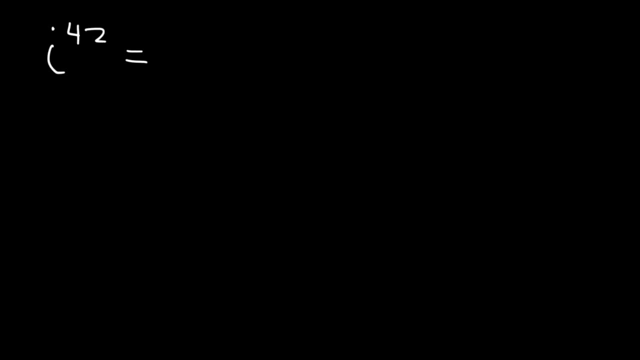 So the highest multiple of 4,, just under 42,, is 1.. So the highest multiple of 4,, just under 42,, is 1.. So the highest multiple of 4,, just under 42,, is 1.. 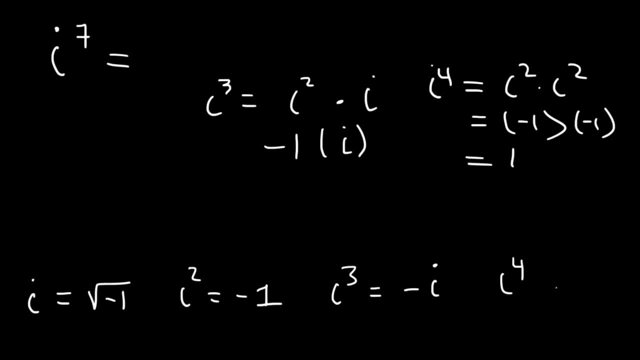 And i squared is negative 1.. Negative 1 times negative 1 is 1.. So i to the 4th is 1.. Make sure you know these four values. The ones that you're going to be using are i squared, i cubed and i to the 4th. 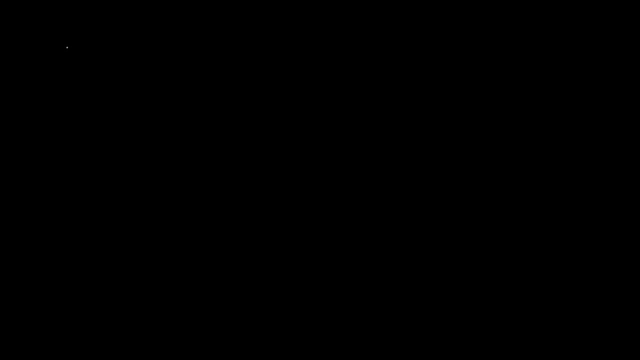 So now let's simplify: i to the 7th power, i to the 7th is i to the 4th times i to the 3rd, Because 4 plus 3 adds up to 7.. Now we know that i to the 4th is 1.. 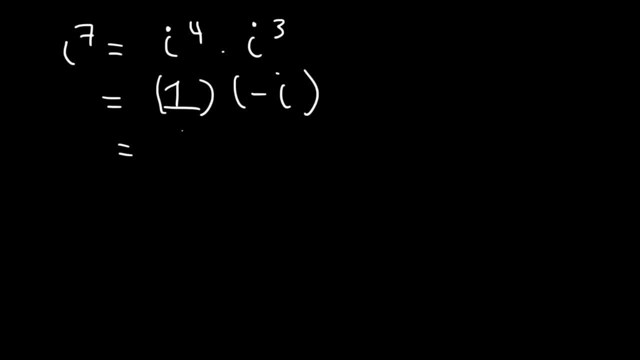 And i to the 3rd is negative. i Therefore i to the 7 simplifies to negative. i Try this one Simplify. i to the 21st power. Feel free to pause the video and work on this example. So this is i to the 20th times. i to the 1st power. 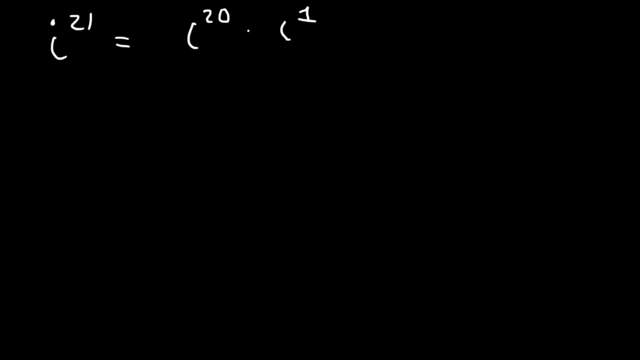 Now, the reason why I chose to separate into 20 and 1 is because 20 is a multiple of 4.. In fact, it's the highest multiple of 4, just under 21.. This one, one of them. you want it to be anywhere between 1 and 3.. 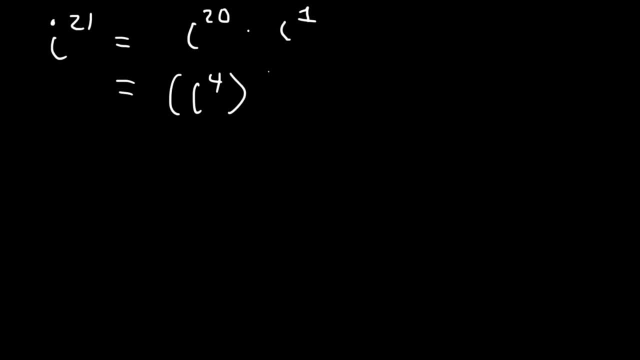 Now, i to the 20th is basically i to the 4th. i to the 4th raised to the 5th power, because 4 times 5 is 20.. And i to the 4th, we know it's 1.. 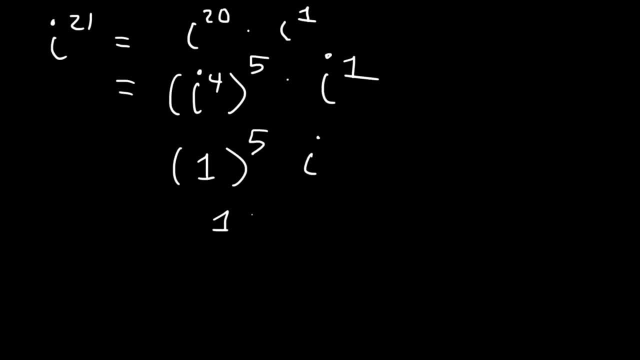 And 1 to the 5th power is simply 1.. So the answer is 1 times i, which is equal to i, And so that's the answer. Here's another one that you could try. Try i raised to the 42nd power. 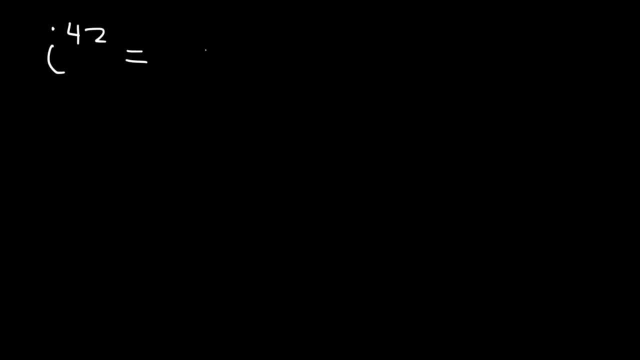 So the highest multiple of 4, just under 42, is 40.. 40 is divisible by 4.. And 40 plus 2 is 42.. If you want a step-by-step process to find out what two numbers to choose from, 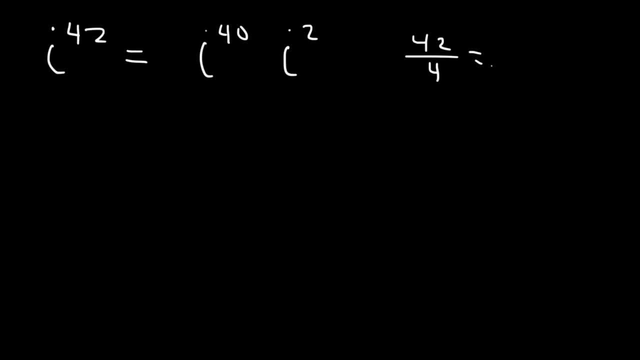 take 42 and divide it by 4.. If you type this in your calculator, you're going to get 10.5.. Multiply 10, the whole number part of 10.5, by 4.. This will give you the first number, 40.. 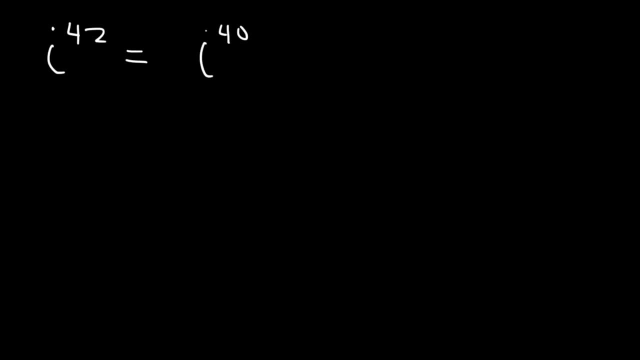 So the lowest multiple iserted to 1 is 40.. 40 is divisible by 4.. And 40 plus 2 is 42.. If you want a step-by-step process to find out what two numbers to choose from, to find out what two numbers to choose from, 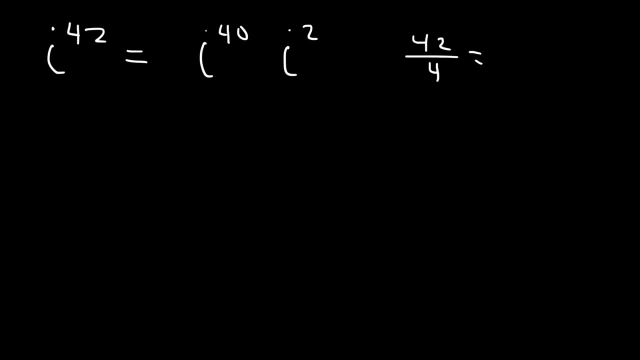 take 42 and divide it by 4.. If you type this in your calculator, you're going to get 10.5.. you're going to get 10.5.. Multiply 10,- the whole number, part of 10.5, by 4.. 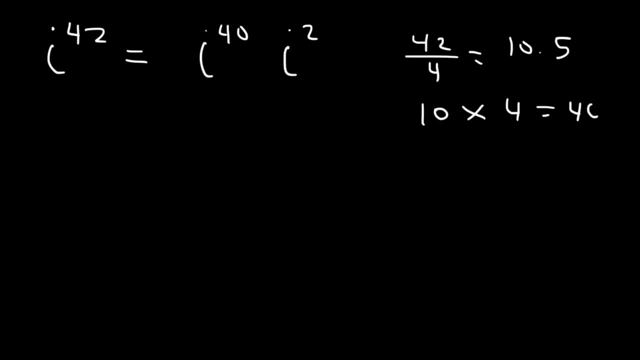 Multiply 10, the whole number part of 10.5, by 4.. This will give you the first number, 40.. And then take 10 and multiply it by the decimal part of this number, which is 0.5, and this will give you 2.. 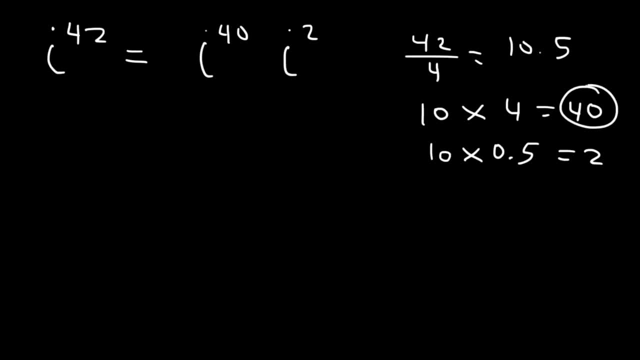 And so you want to separate 42 into 40 and 2.. Now i to the 40 is basically i to the 4th raised to the 10th power. So if you take 40 and divide it by 4, you're going to get this number 10.. 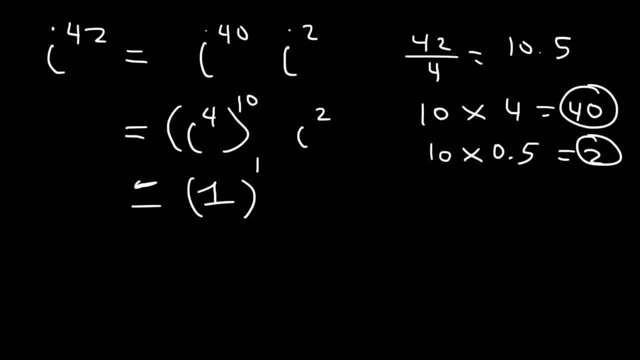 i to the 4th is basically 1, and i squared is negative 1.. 1 to the 10th power is 1.. 1 times negative, 1 is negative 1.. So that's the final answer. What about this one i raised to the 189?? 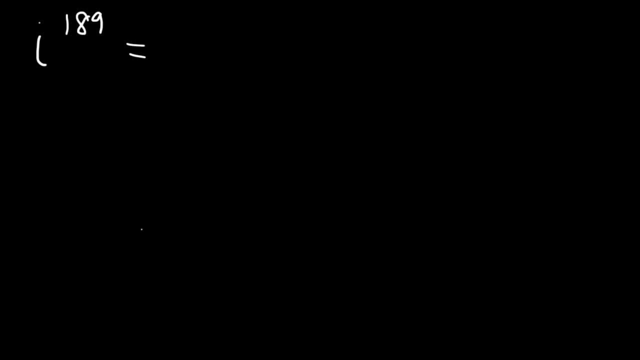 Go ahead and simplify that example. So let's start by dividing 189 by 4.. This is equal to 47.25.. Now take the whole number portion of 47.25, which is 47. And multiply that by 4.. 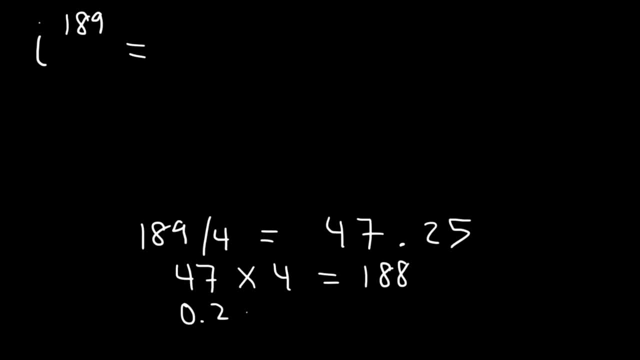 So that's 188.. And if you take the decimal portion and multiply it by 4, you get the remainder, which is 1.. So let's decompose it into 188 and 1.. Now 188 divided by 4 is going to equal 47.. 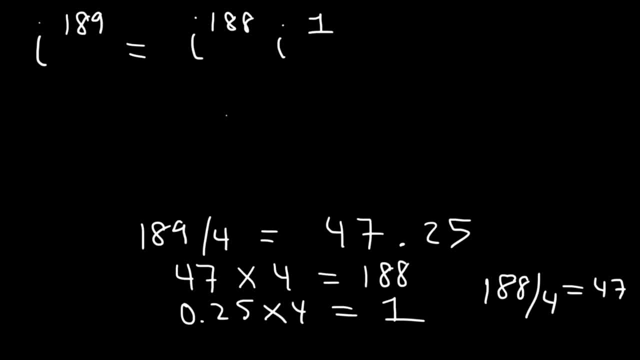 Because 47 times 4 is 188.. So what you want to do is You want to break down 188 into i to the 4th, raised to the 47th, And you know, i to the 4th is 1.. 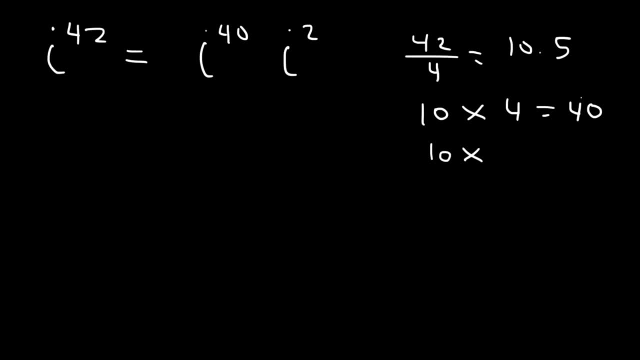 And then take 10 and multiply it by the decimal part of this number, which is 0.5. And this will give you 2.. And so you want to separate 42 into 40 and 2.. Now i to the 40 is basically i to the 4th raised to the 10th power. 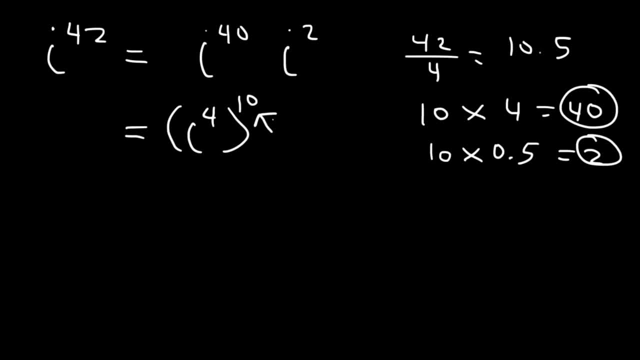 So if you take 40 and divide it by 4, you're going to get this number 10.. i to the 4th is basically 1. And i squared is negative 1.. 1 to the 10th power is 1.. 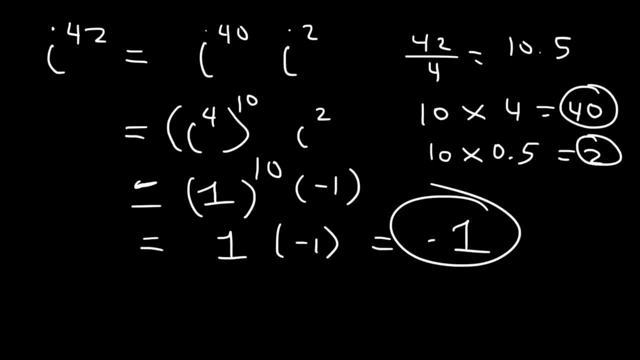 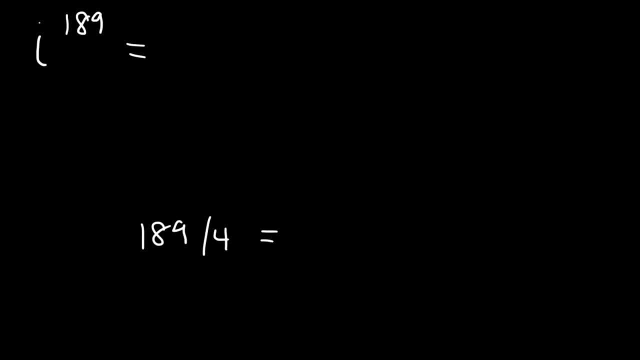 1 times negative. 1 is negative 1.. So that's the final answer. What about this one i raised to the 189.. Go ahead and simplify that example. So let's start by dividing 189 by 4.. This is equal to 47.25.. 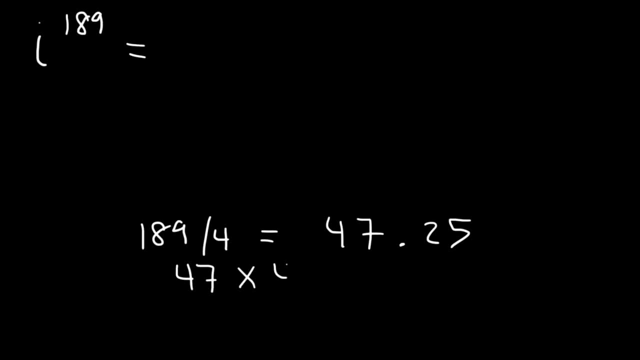 Now take the whole number portion of 47.25, which is 47. And multiply that by 4.. So that's 188.. And if you take the decimal portion and multiply it by 4, you get the remainder, which is 1.. 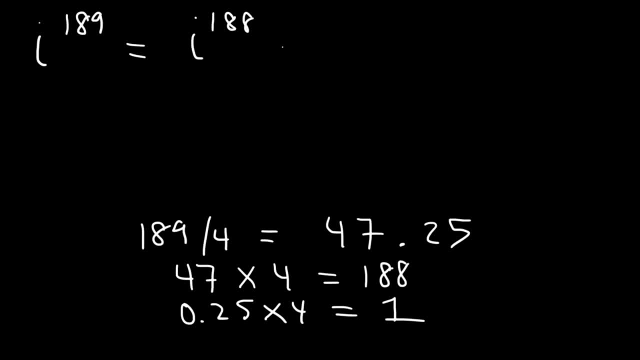 So let's decompose it into 188 and 1.. Now, 188 divided by 4 is going to equal 47. Because 47 times 4 is 188.. So what you want to do is you want to break down 188 into i to the 4th, raised to the 47th. 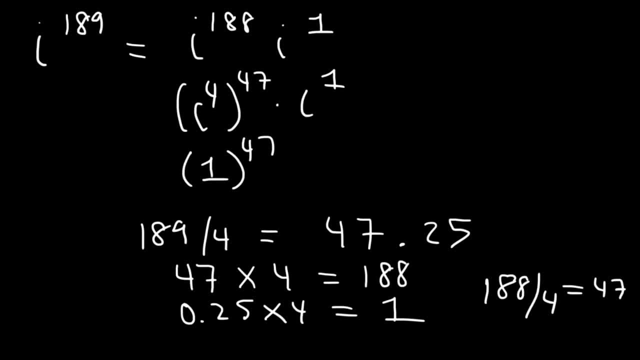 And you know, i to the 4th is 1.. And 1 to the 47th is simply 1.. So this becomes 1 times i. So the final answer is: i Go ahead and simplify this expression: 3i raised to the 8th, minus 4i to the 13th. 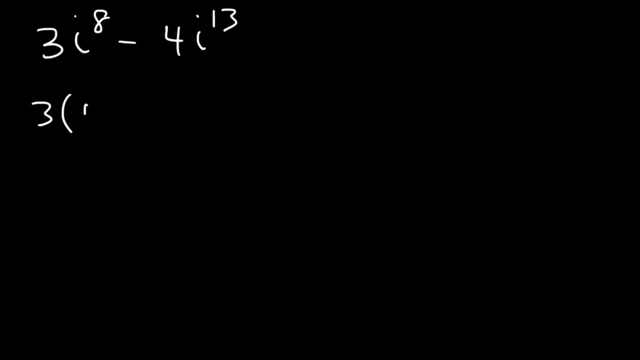 So 8 is a multiple. I'm going to write it as i to the 4th squared, Because 4 times 2 is 8.. Now 13,. we can break it into 12 and 1.. i to the 4th is 1..